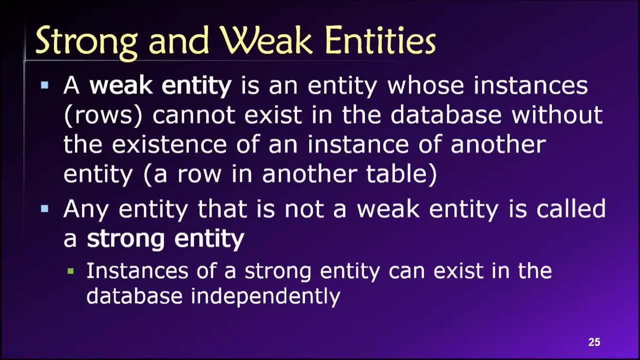 various entities that collectively represent the tables in the database, and we have the relationships between them, the cardinalities and so on. Among all of those entities, we can classify each one as either being weak or strong. So the difference between a weak and 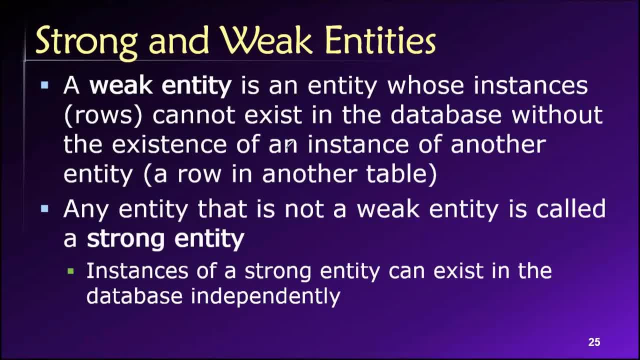 a strong entity is simply this: Can we add new rows of data to that entity or to that table without there already being some kind of matching relationship? So if an entity is weak, which is described by this major bullet point, what that means is that we cannot add any rows to that table unless matching or related rows exist in another. 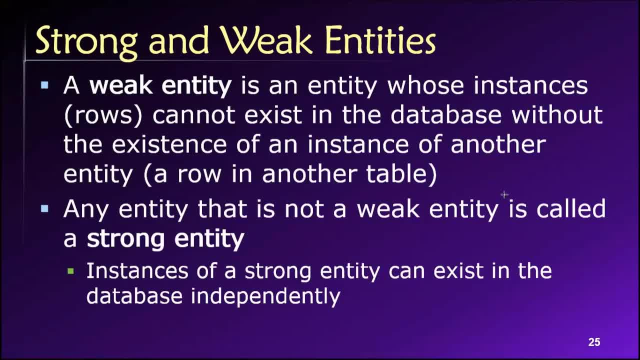 table. Any entity that is not weak is, by definition, strong. So with a strong entity we can add new rows to the table regardless of whether there are any matching or related rows in some other table. So that is the instances of a strong entity can stand. 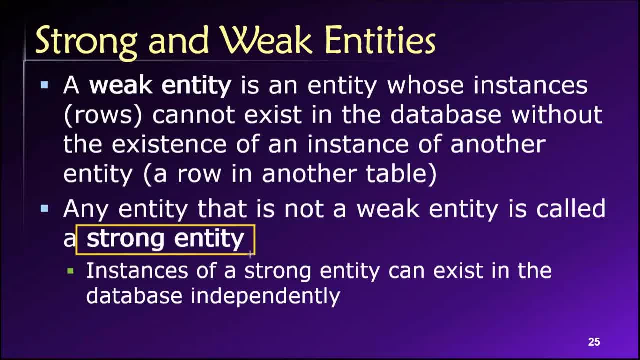 or exist on their own in the database without having any sort of connection to or reliance upon another entity for their existence, And also note that it's perfectly feasible for instances of a strong entity to exist in another entity, So we can add new rows to the table without 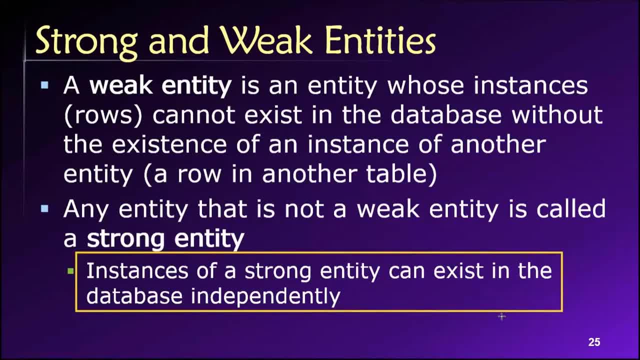 exist independently in a database, meaning that they don't have any relationships, right? So I can have it like an unrelated table. That would be a strong entity. And I can also have entities that are related to other tables but are nevertheless strong. 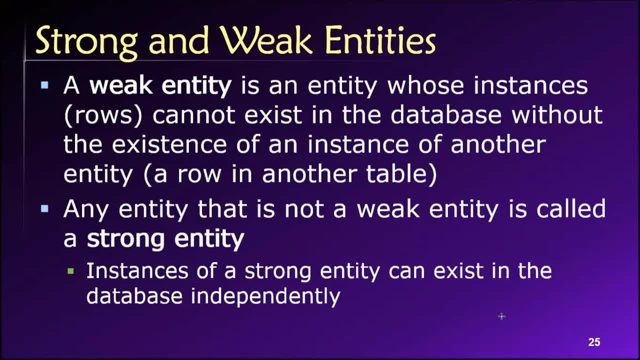 because it's possible to add rows to those tables. They're needing to be some sort of matching or related row in another table. Okay, So strong versus weak entities. Let me very briefly switch over to our now very familiar employees database that we've 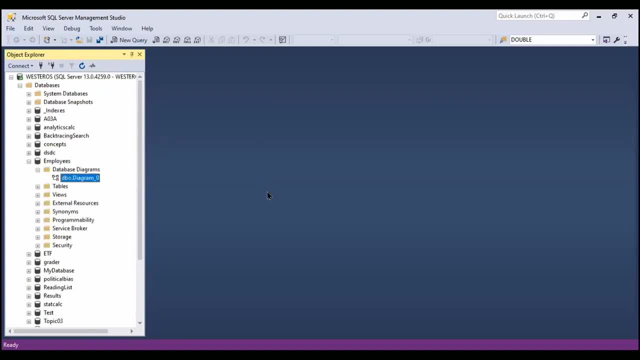 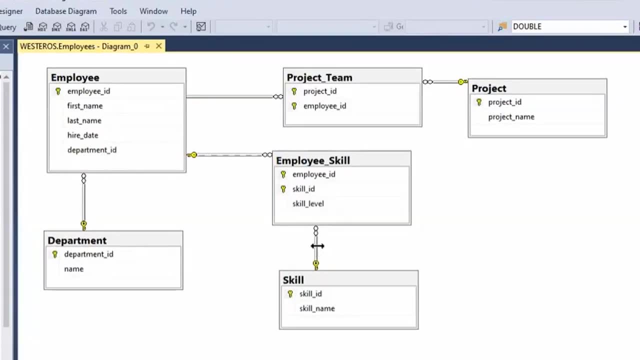 been tinkering with, And with that notion in mind of strong versus weak entities, we can now look at this simple database diagram out here and ask ourselves which of these entities is strong and which of them may be weak. So remember a strong entity. 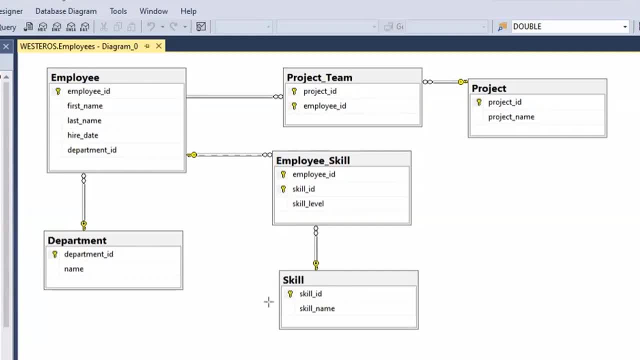 And if you look at this table, you can see that a strong entity can exist in the database without the necessity of a relationship. So if I look out here and I ask myself this question: like, could I add a new row to this skill table? 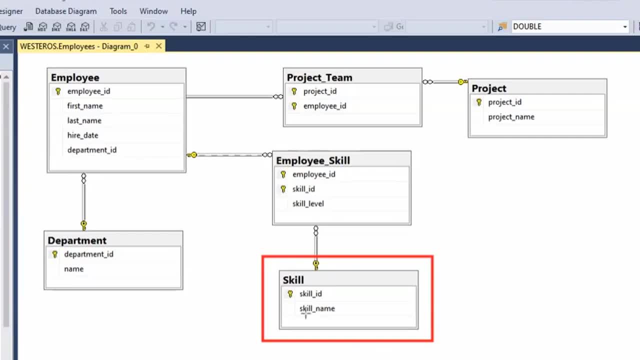 without there being any matching rows in another table, And the answer, of course, is yes, I could have a new skill right. Maybe my new skill that I want to measure for my employees is their- I don't know their- ability to type. 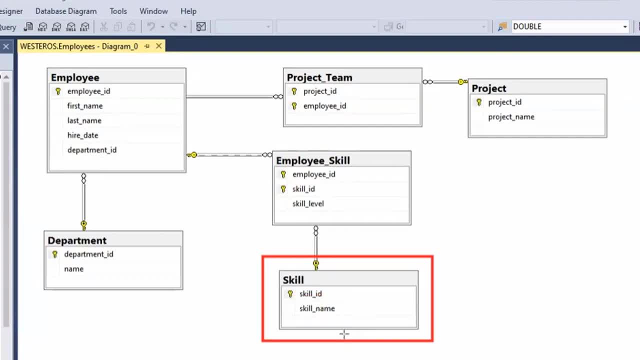 Okay, So I could add that as a new skill to the skill table without there being any other rows in a connected table that are associated with typing. So a skill table here would be a strong entity. Similarly, we could add departments, right. 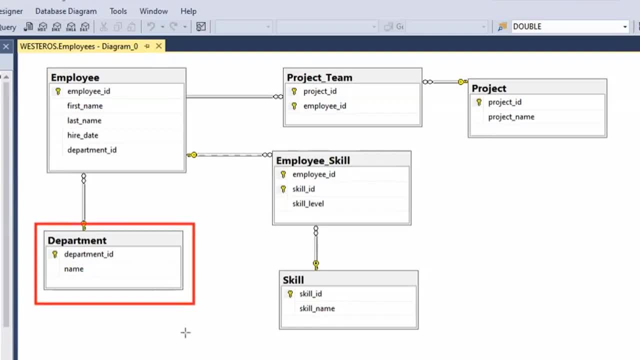 So we can have additional departments. We can add as many as we need without there being any related employees. So department is a strong table right, Project is a strong table right. I could add new projects to this project table without to there being any related rows anywhere else. 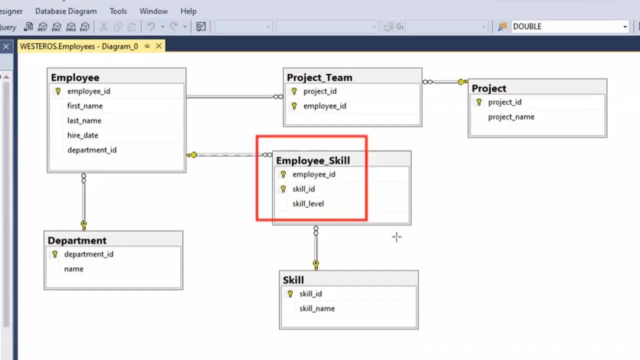 So then we can take a look at some of these other tables, like employee skill right. In this case, in order for a row to be added to this table, there must already be a matching skill ID in the skill table down here. So then we can see that, because this is part of the primary table, 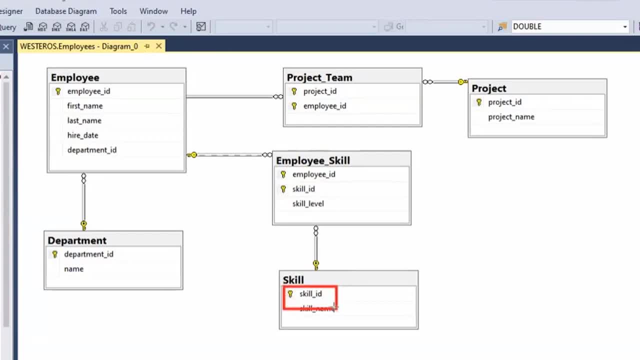 So we can see that because this is part of the primary key right And it's also a foreign key which connects us down here. So that means I cannot add a new record to this employee skill table unless the skill ID for that new record already. 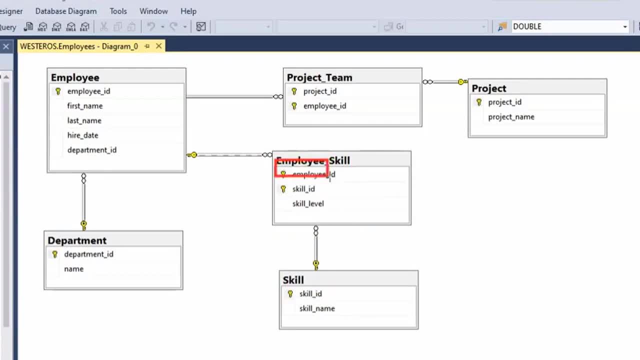 exists down here in the skill table, And the same applies to the relationship between employee ID and employee ID over here. So employee skill is definitely a weak. we can't add any new rows to the employee skill table unless we already have appropriate matching rows. 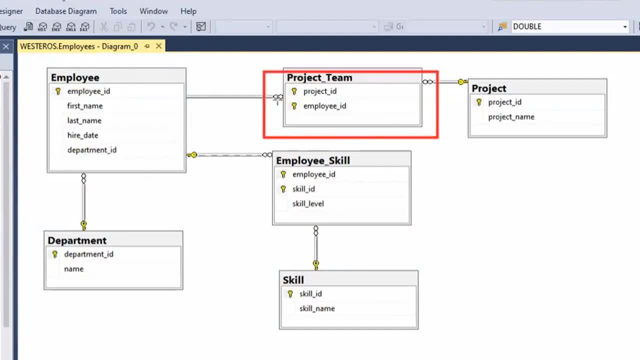 Here and here- and the same thing applies with this table here. right, We need to have existing projects and existing employees in the related tables in order to add new rows to this table. So this would be a weak entity as well. And then we have an interesting question, and that is: is the employee entity strong or weak?